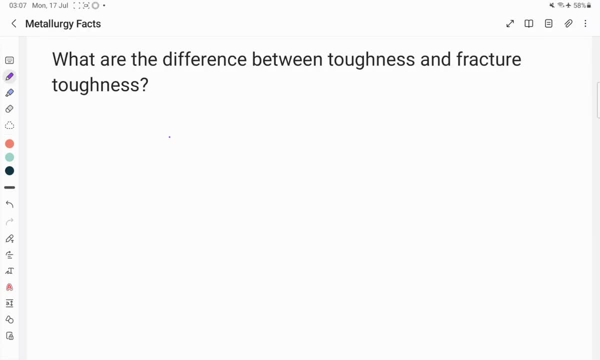 hello everyone, welcome to our YouTube channel, metallurgical engineering. so in this video we are going to see the difference between toughness and fracture toughness. so toughness and fracture toughness are both mechanical properties, both are the mechanical properties. so basically this describes the materials resistance to fracture. so they have distinct definitions, so both 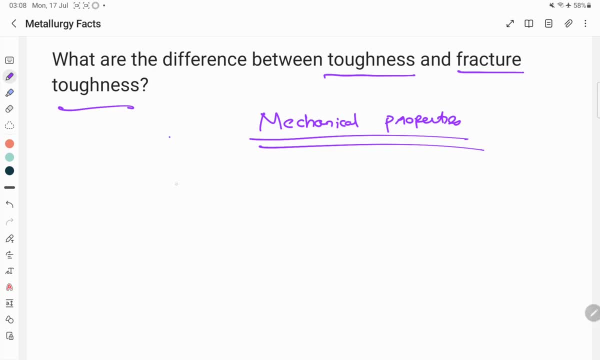 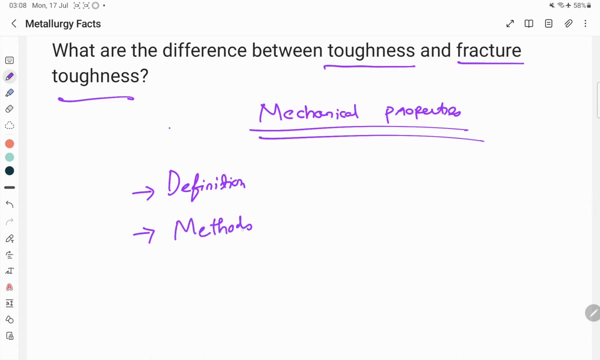 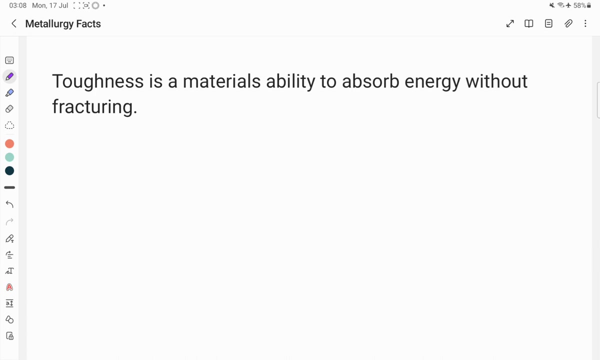 has distinct definitions as well as applications. so in this video we are going to see the definition of both toughness and fracture toughness and then- and then this- we will see the methods by which we can determine this toughness and fracture toughness, and also some applications, different applications. so let's start the video. so now, the first term is a. 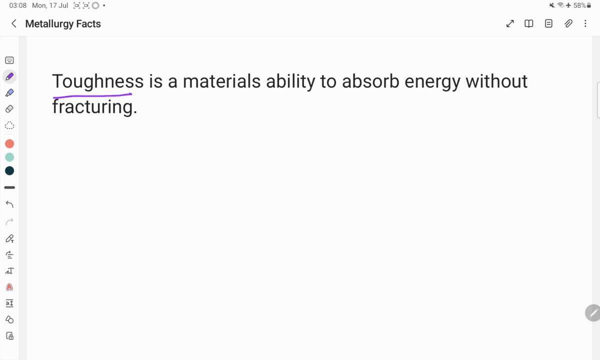 toughness. so basically it is a materials ability to absorb energy without fracturing. so toughness is a combination of, if you will see this toughness it is a combination of strength plus ductility. so it it is typically determined by two methods, so that two method we are going to see here. so the first one is tensile. 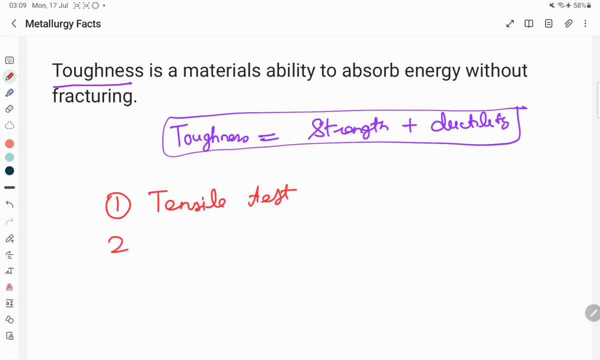 test. the second method is impact test. so we will see both here. so first one is tensile test. so the output of this tensile test is stress versus strain diagram. so on the y-axis we have a stress and on the x-axis we have a strain here. so basically, here we are talking about engineering: stress versus. 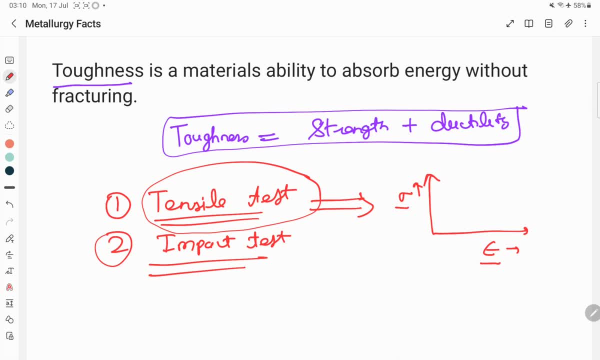 engineering strain. so if we can take an example of aluminium so, which is a ductile material, so the stress versus strain of aluminium is usually looks like this. so this has two parts. the first one is elastic region and the second one is elastic region. so the area under this elastic as well as this. 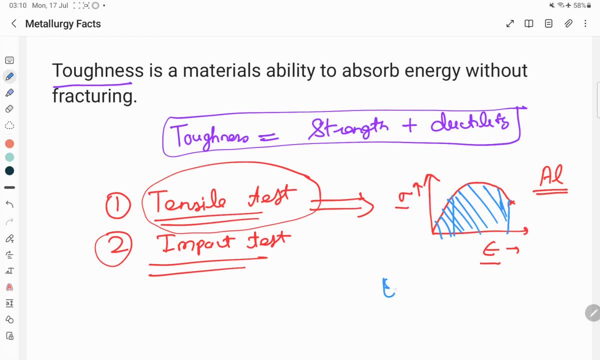 plastic region is known as toughness, elastic plus plastic that we call as. the area under this is called as toughness, so you can measure a toughness using this, this tensile test, while the area under this elastic curve it is known as resilience, resilience. okay, so now we will go this move to the second one with this, which 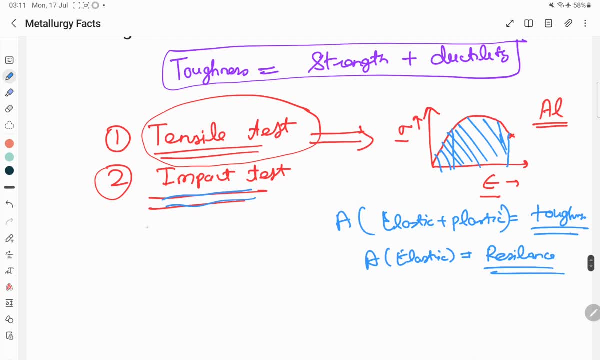 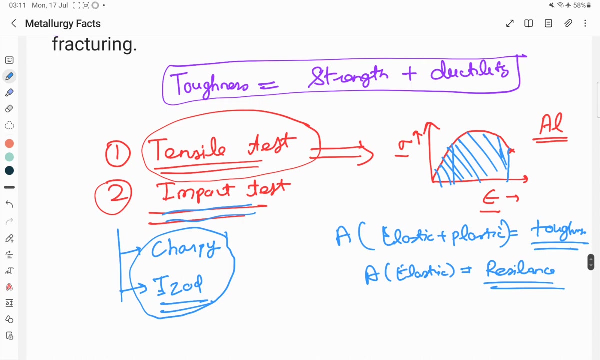 is called impact test. so basically, this impact test can be done by two way. the first one is will do the Charpy and the second one will do IZOT. so these two tests can be used to determine the toughness of any of any this, this material. now, if you are going to do this, 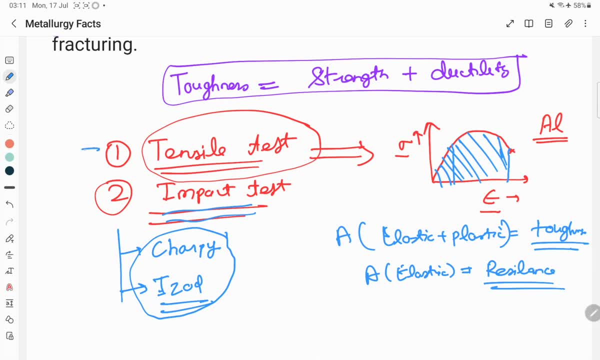 tensile test and impact test, so you have to follow some ASTM standards. so, basically, if you are dealing with this metallic material, so for a tensile test you you can use ASTM E8 or E8M standards and for impact tests you can use ASTM E23 for preparing the specimens for tensile and impact test. now we'll go. 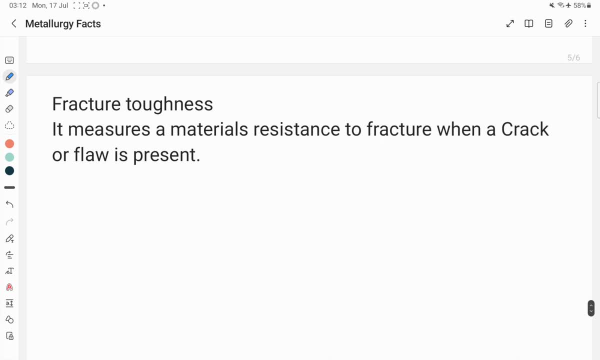 to the fracture toughness. so fracture toughness it tells about the this, about the materials: resistance to fracture when a crack or flaw is present. so basically, if you have any material like this and you can prepare some notch here and then give some pre cracking here and then apply a load here like this, so how much energy is absorbed? 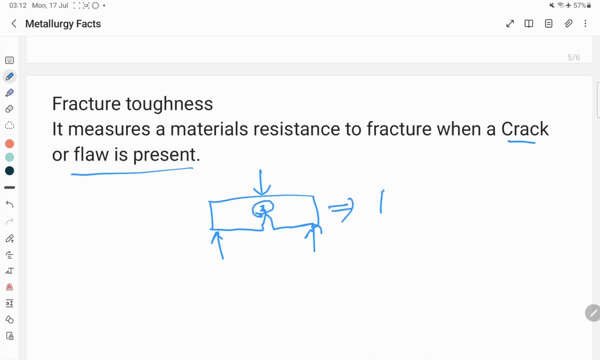 in presence of crack. that will tells the idea of fracture toughness. so the difference, the main difference between fracture toughness and toughness is that in fracture toughness the flaw or the crack is present and then you are seeing how much energy is absorbed. but in case of toughness there is no crack and flaw.